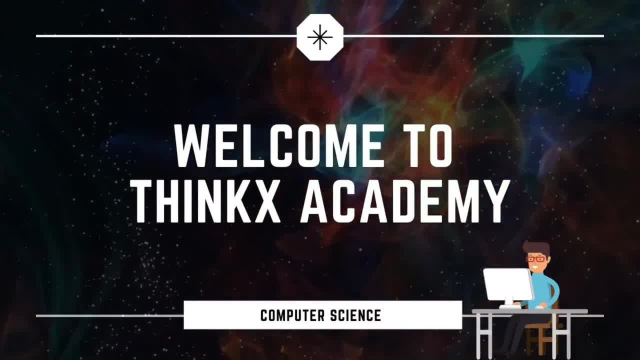 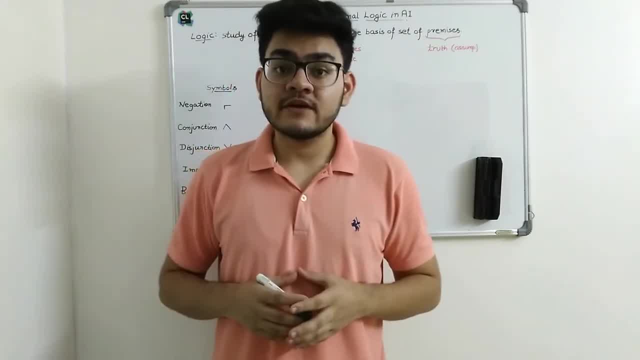 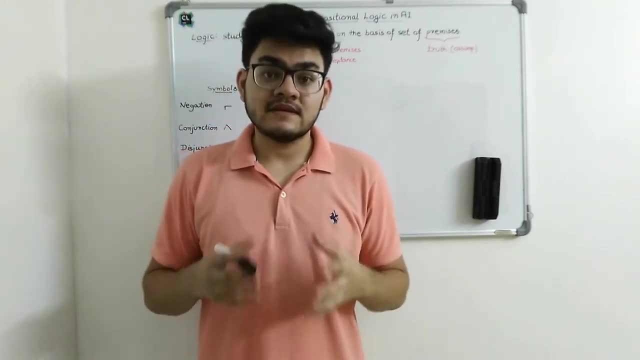 Hi Thinkers, welcome to the artificial intelligence playlist on ThinkX Academy. In this tutorial we are going to start with propositional logic in artificial intelligence. So basically, in this series, in this playlist of artificial intelligence, we have already covered a lot of algorithms like hill climbing. 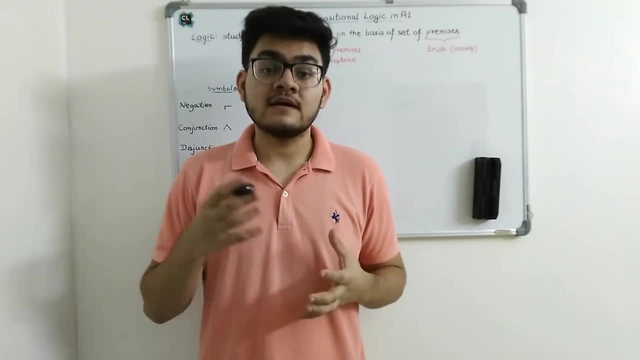 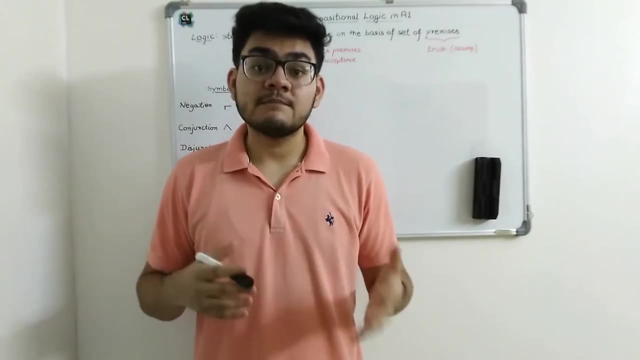 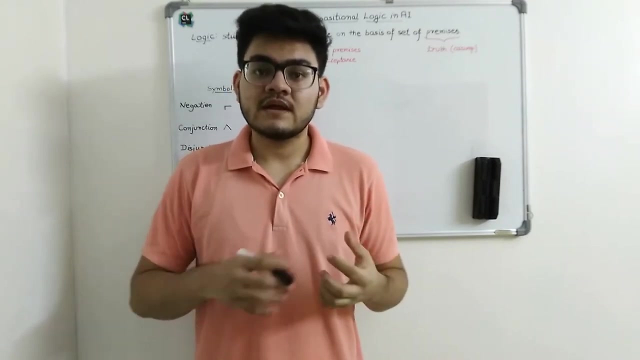 Then we have studied about heuristics and alpha beta pruning, best first search. We have studied a lot of algorithms where basically we have also covered game playing algorithms also. So basically we know that how an AI works is by starting with some node and going to a goal state, finding the best path. all of that. 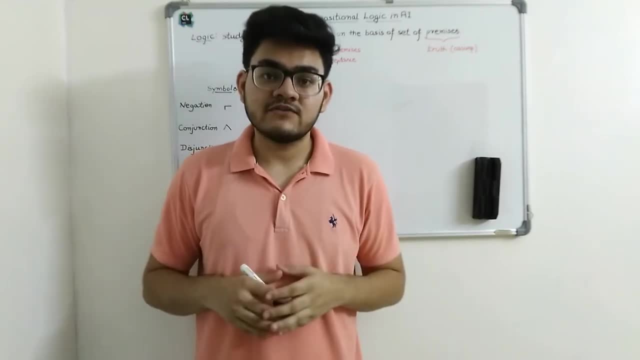 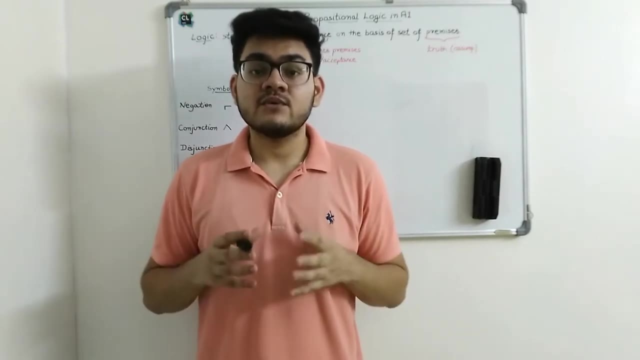 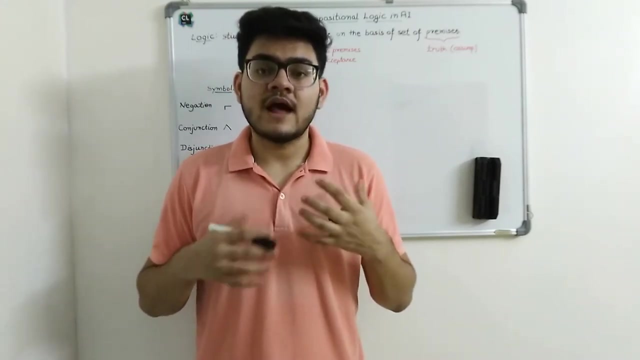 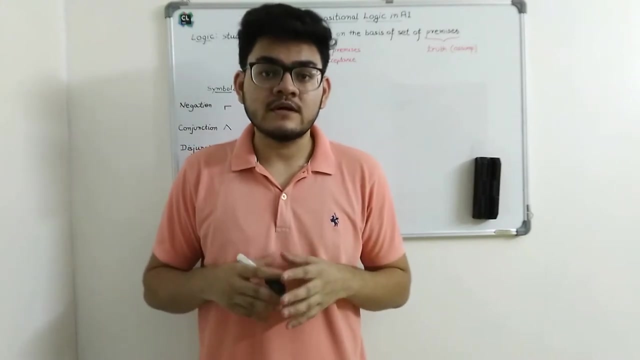 That comes in the first phase, or first side of artificial intelligence. There is a second phase of artificial intelligence Which is very important, which is known as reasoning and logic. Reasoning and logic: just like we humans, we have some knowledge And according to that knowledge we form some of our logics, which may be true or not, but there are some logics which we make in our daily lives. 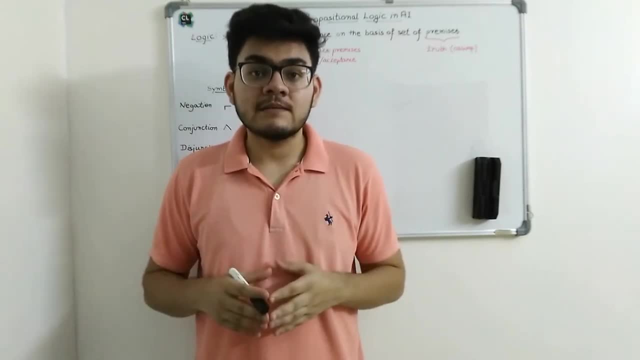 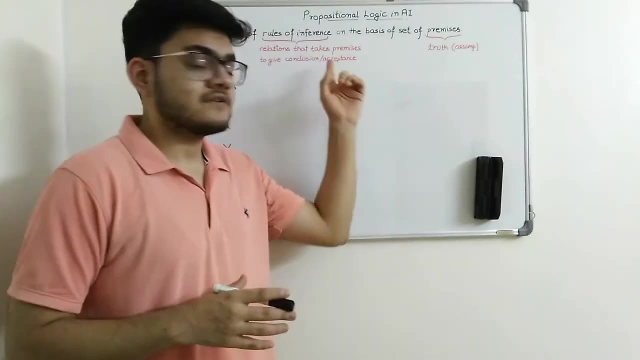 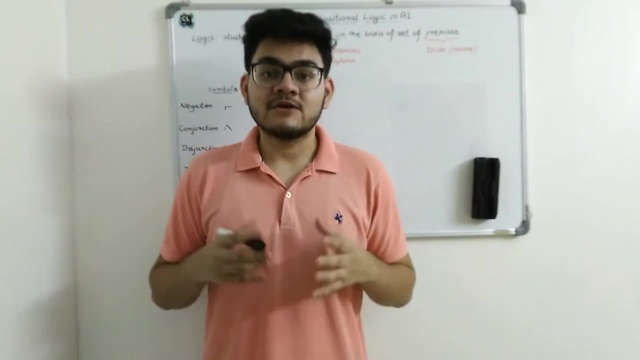 Similar to that. the AI systems are also capable of making these types of logic. So we are going to start with very simple logic systems, Which is the propositional logic. So, before starting with the video, make sure to like this video and subscribe our channel, because I keep creating this awesome free content for you guys. 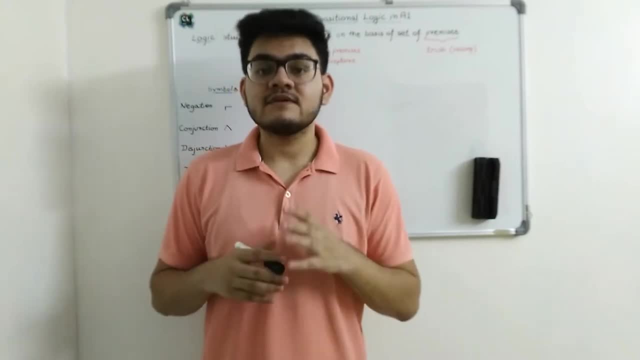 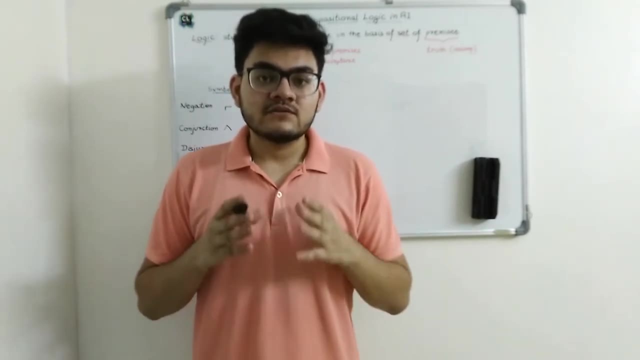 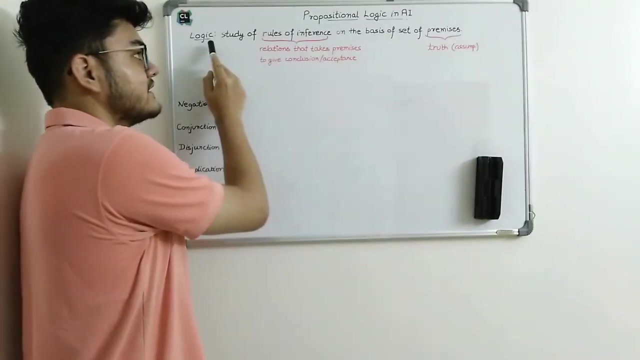 So now let's get started. The first thing we need to understand before understanding propositional logic is what exactly is a logic? So I'm going to give you a very formal definition of logic here. So here I have written the logic definition, which says that it is the structure. 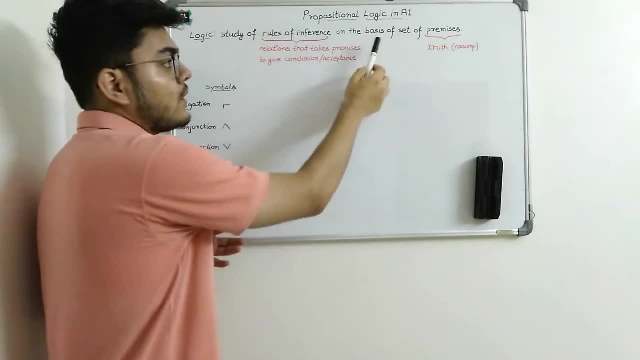 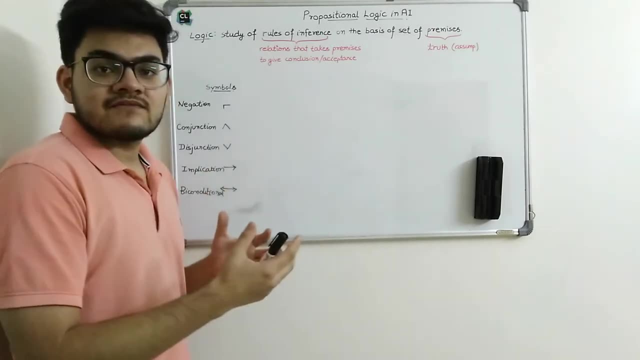 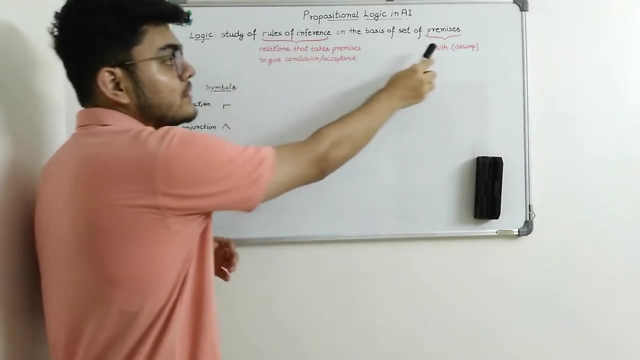 It is the study of rules of inference on the basis of set of premises. So this is the formal definition. So let's break down this definition, Let's try to understand what exactly is a logic. So here you can see we have two important terms, which is premises and rules of inference. 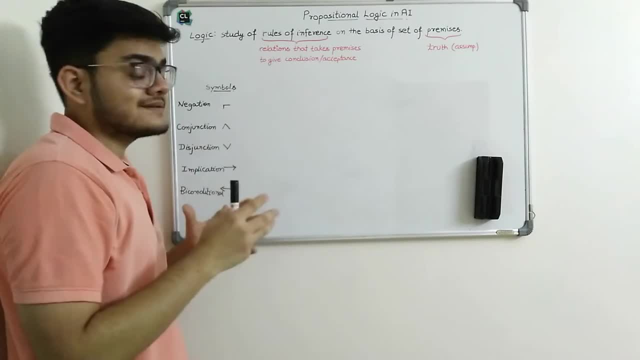 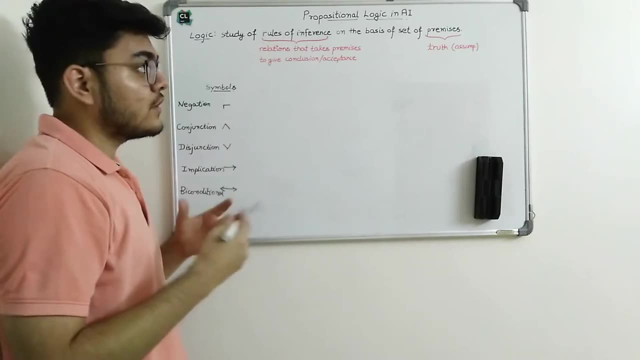 These are very important terms And at this point understanding what exactly is a logic is very important Because in the further study Coming tutorials they will cover a lot of things related to propositional logic And there is another one which is the predicate logic. 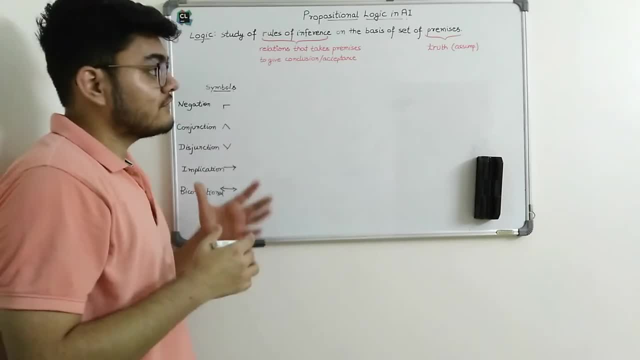 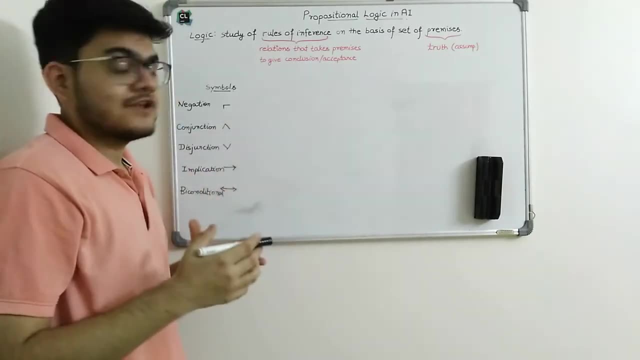 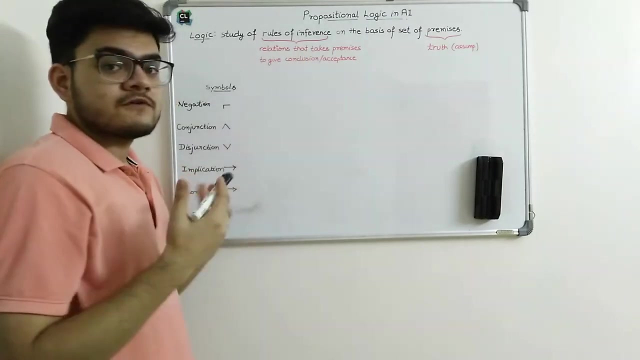 And we also have a logic programming language for AI, which is prologue programming. So it is essential that at this point, you focus on this very important definition here. So it is the study of rules of inference. What is the rules of inference? 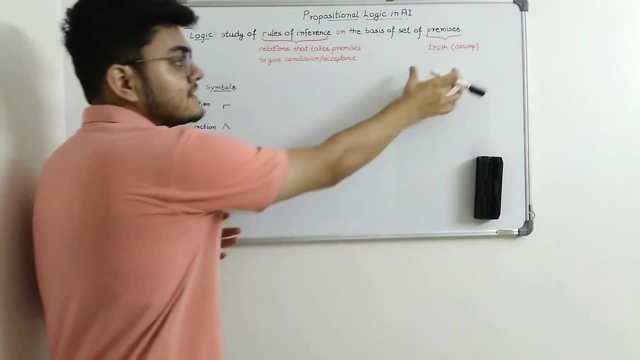 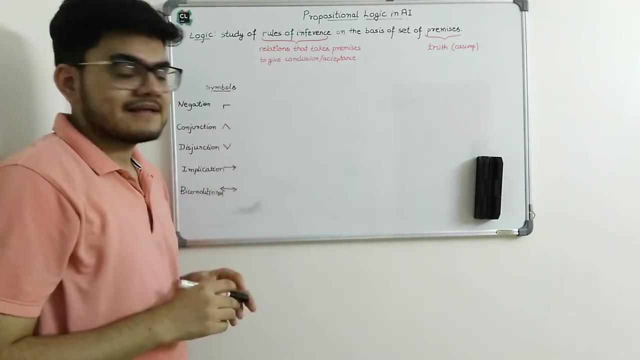 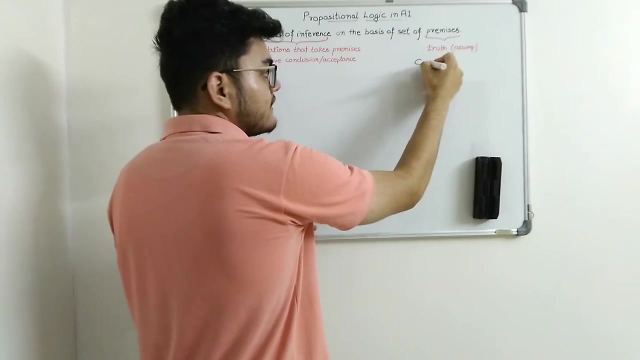 I have written here. It is the set of definitions that takes premises to give some conclusion. So I am going to explain this with the help of a very simple example here. So let's say there is a company A And let's say- I have a very simple example here- that there is a company A. 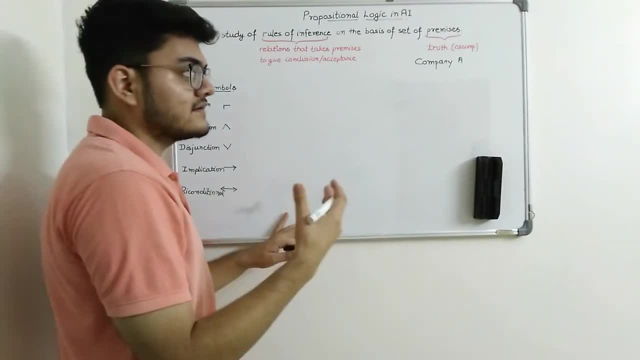 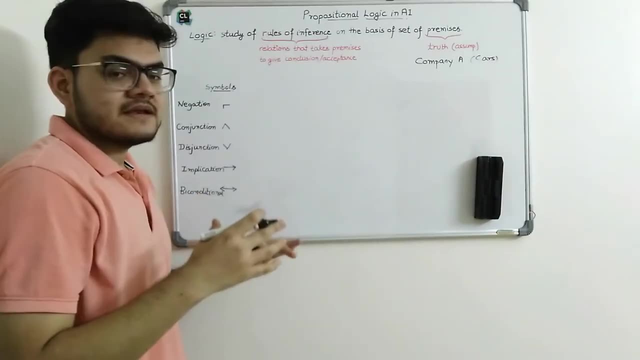 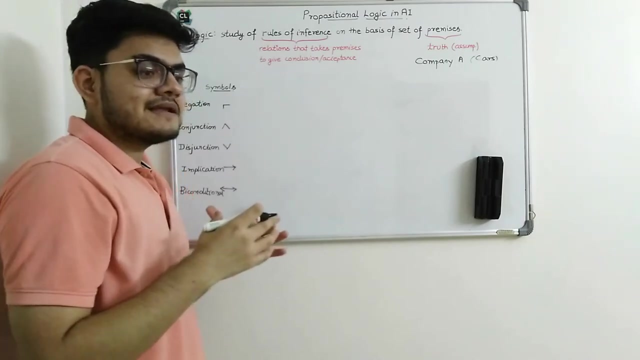 And let's say, this company actually deals with automobiles, like cars and all of that stuff. So what is premises? It is basically truth. All the statements that actually reveal some truth, statements And basically, whether they are truth or not, it is an assumption that it is a truth. 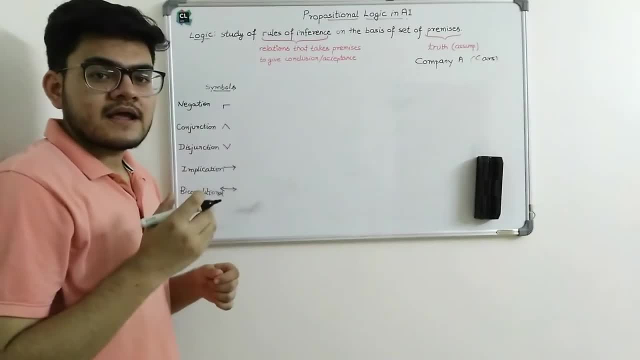 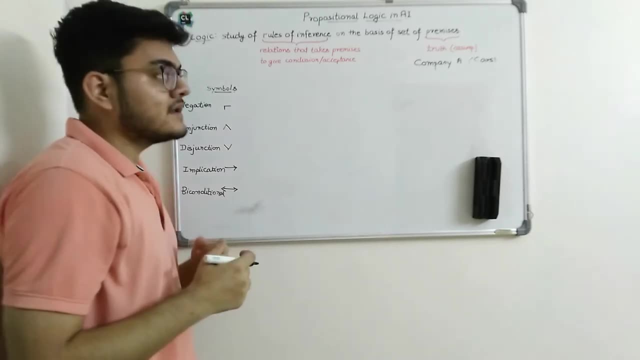 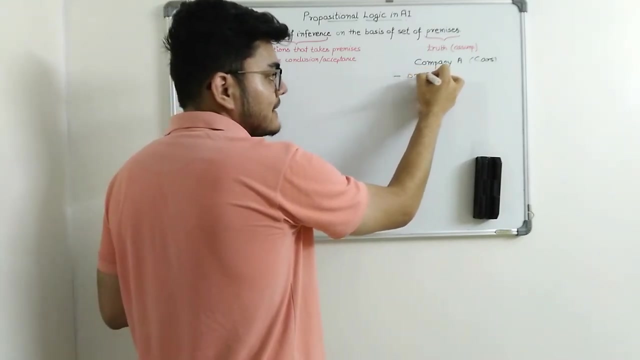 So let's say we have a company A And I have some knowledge, or we can say some statements which are true, about this company. So let's say that I have some knowledge about this company And the production in this company is going to rise. 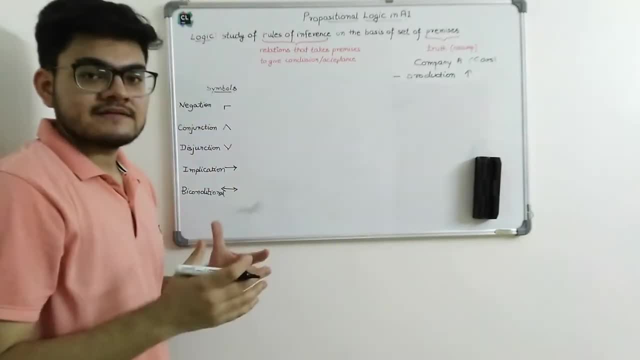 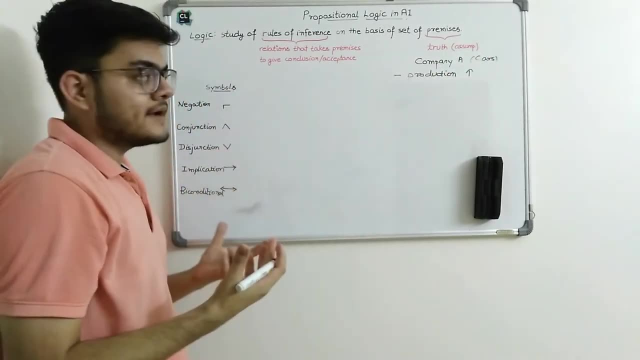 In the next coming week, the production in this company is going to rise. This is one of the truth statements that I am saying here. It is an assumption. Now I have some more truth statements about this company. The first thing is the production is going to rise. 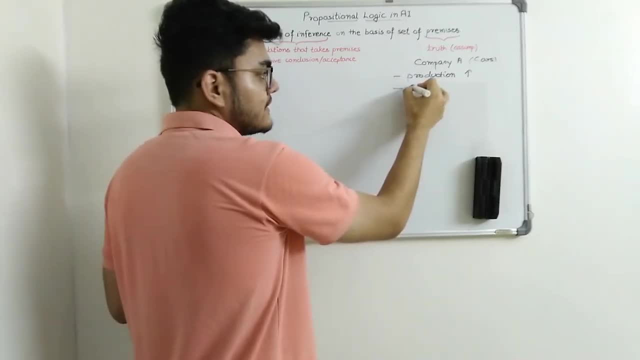 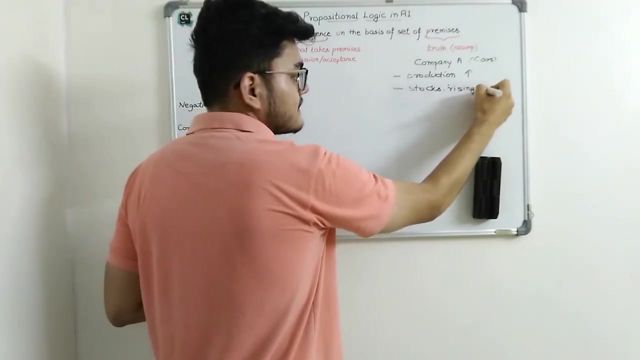 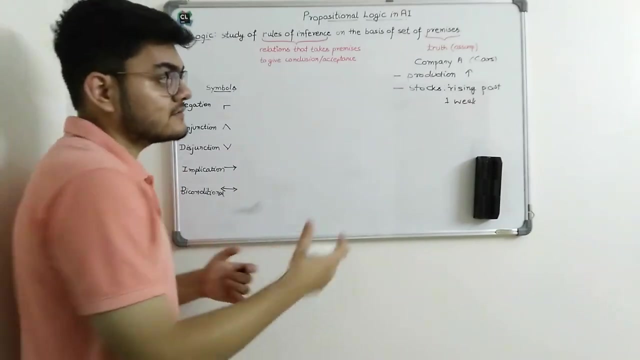 So let's say that we have some more things about this company, More things about this company A, Which is, let's say, the stocks of this company are actually rising for past one week, Right? So the stocks of this company A is also rising past one week. 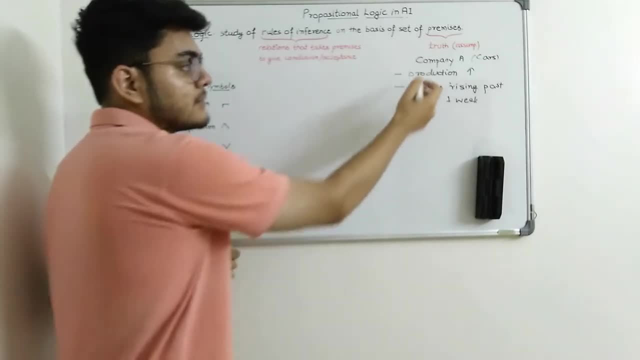 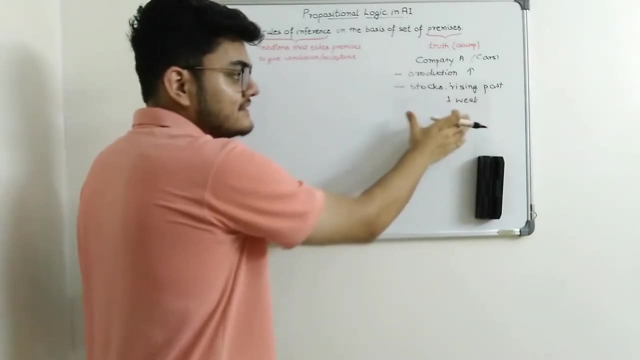 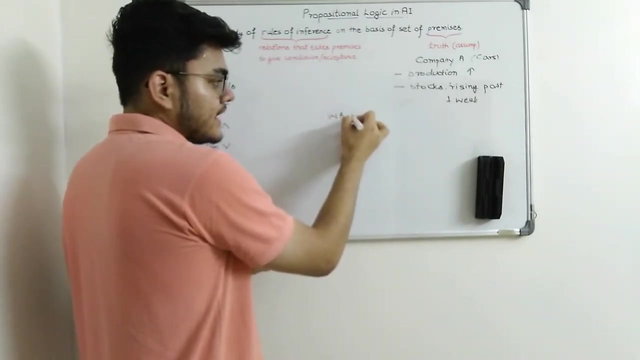 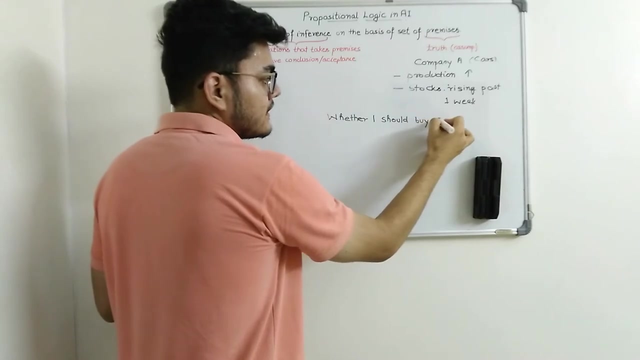 It has a rise in the stocks and the production is also rising. So I have these two statements, These two statements which are true statements. Now, based on these statements, I will have to derive a logic that, whether Right, I am going to write here whether I should buy stocks of the company A. 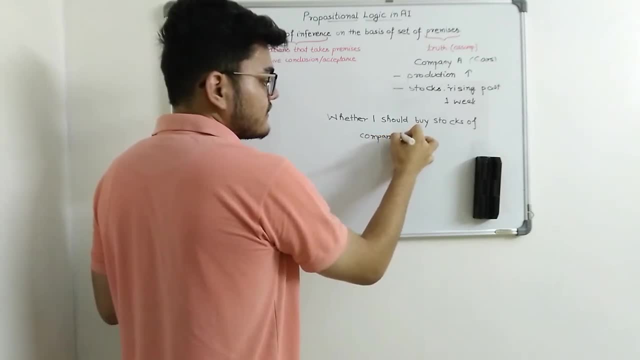 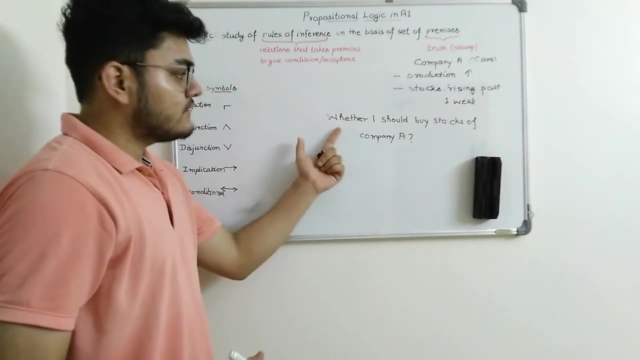 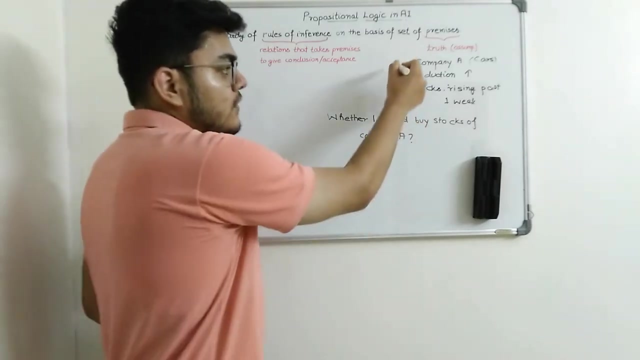 Right? So I have this very simple question here. Right, I have to derive a logic out of this premises, Right? So, whether I should buy the stocks of company A. For that I need two things. The first thing is some of the knowledge, which I believe is true. 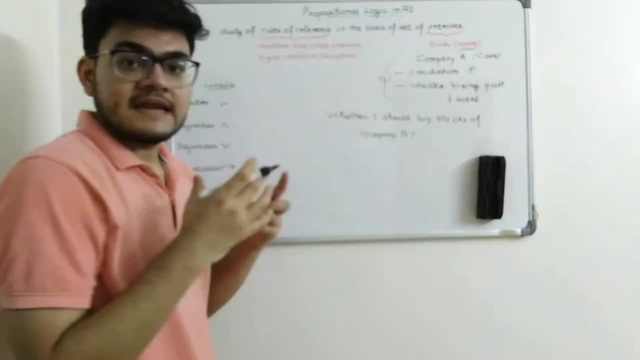 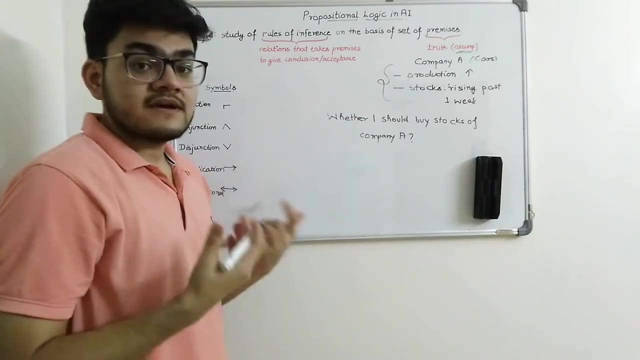 Which I assume to be true. So I need that knowledge to actually derive a logic. Right, That's a very complete traditional way In your real life also, you can relate it That whenever you want to derive a logic, You will first have to. 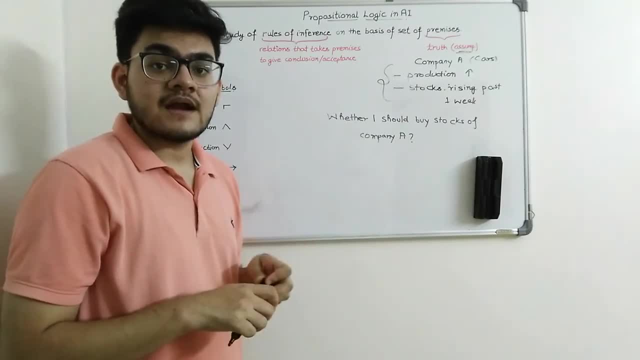 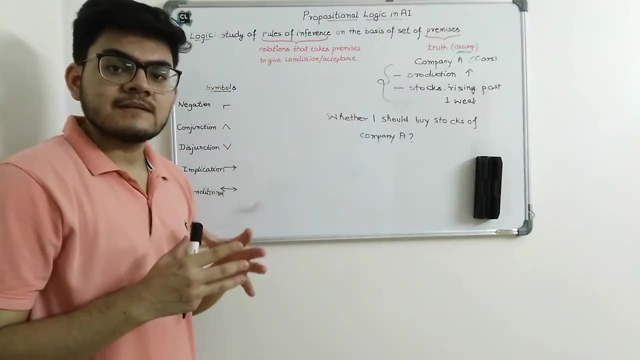 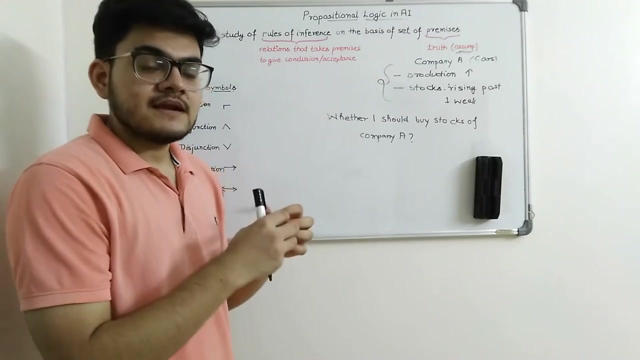 Actually analyze some of the statements and some of the experiences. And the second thing which is important is rules of inference. Rules of inference are basically rules. What it does is it takes this knowledge And then it analyzes that knowledge And then it gives a conclusion. 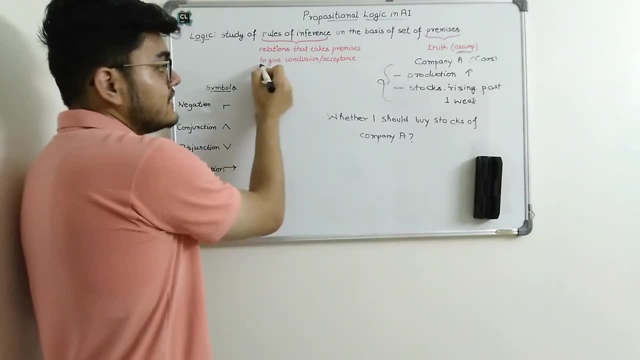 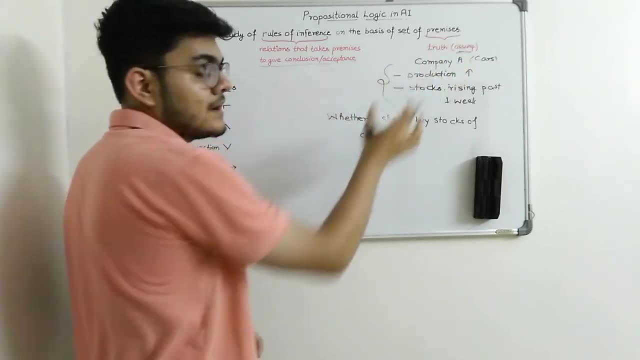 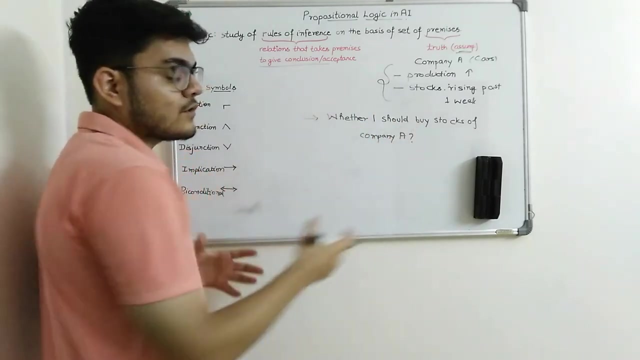 Right. So here you can see. I have written here To give conclusion Right And acceptance. Acceptance of premises. So if I am given some statements, I am going to derive a logic: Whether I should buy the stocks of this company. 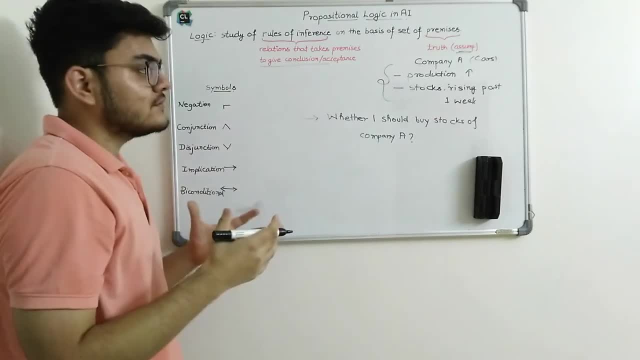 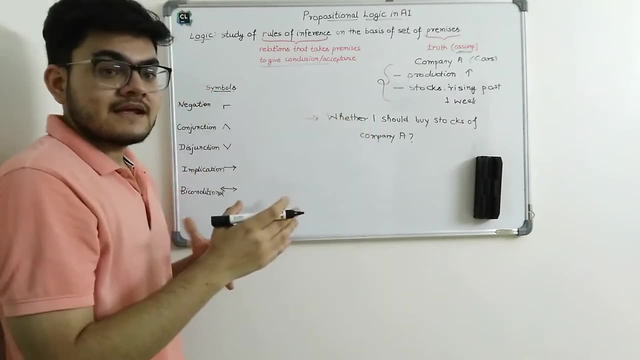 On the basis of some rules, Right. So those rules can be anything. For example, let's say there is a rule which says That if the production of a company is rising And the stocks are also rising past one week, Then you should buy the stocks. 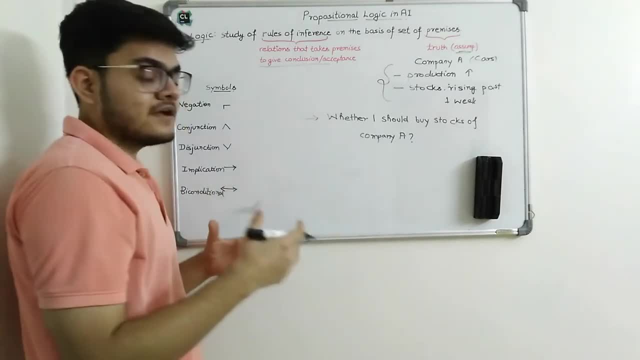 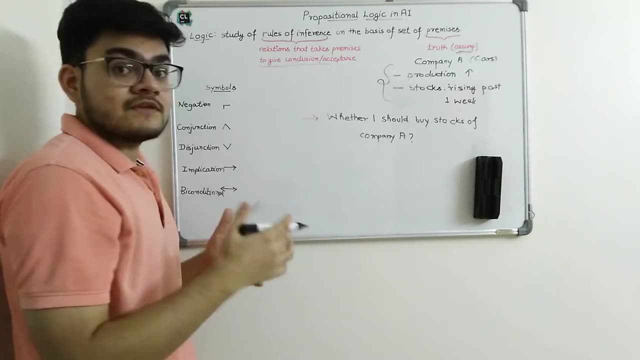 And let's say there is some logic Which says that, Which is contradictory, Which says that the production, If the production is rising, Then even if the stocks is rising past one week, You may or may not consider buying the stocks, Right? 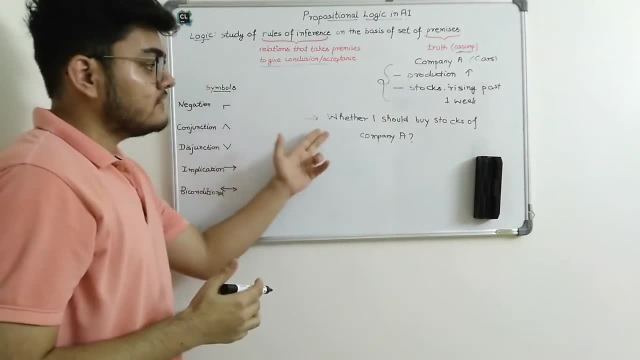 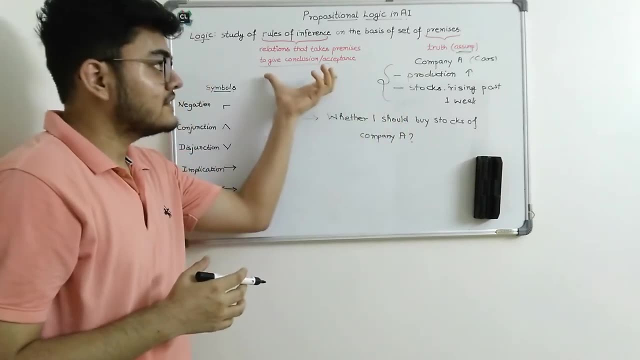 So this is a very important thing. Whenever we want to derive a logic, First we consider premises, Which is basically The statements that reveals the truth, And then we supply these statements To the rules of inferences. Rules of inferences are basically rules. 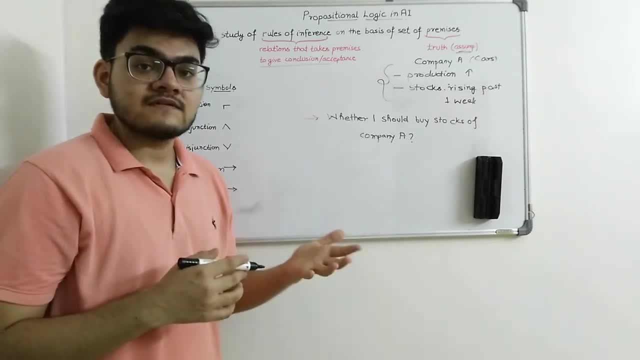 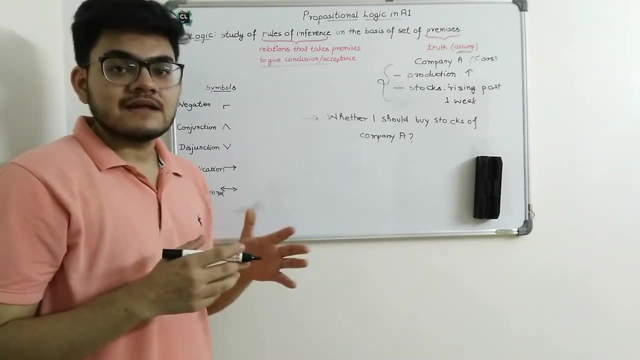 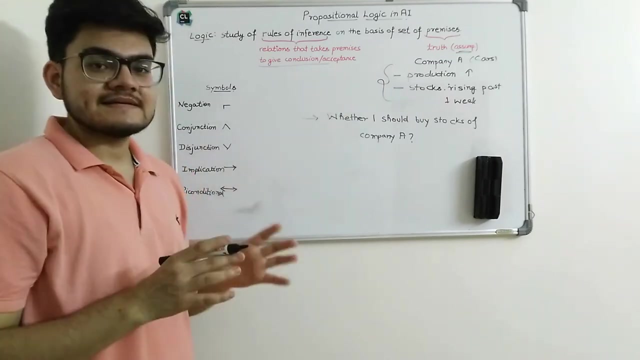 Which give or infer something. Infer means giving a conclusion Right, So they give conclusion. In the upcoming tutorials We will study about Modest ponence law, Which is actually a rule of inference only. So basically, this is a very 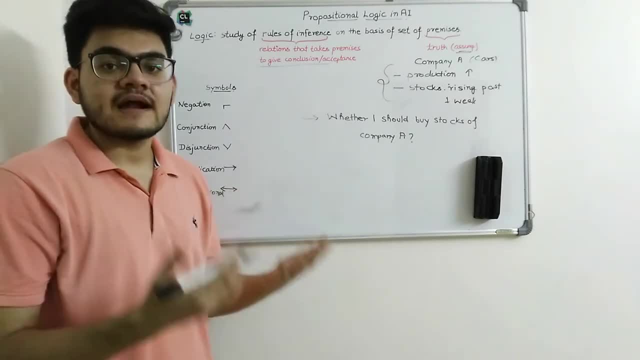 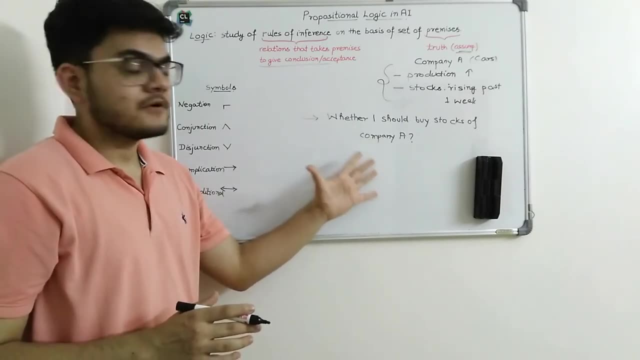 You can say A simple explanation of what exactly is a logic, So I hope you have understood At this point what is a logic. It is crucial to understand this point Because The rest of the AI course will include All the different types of logic. 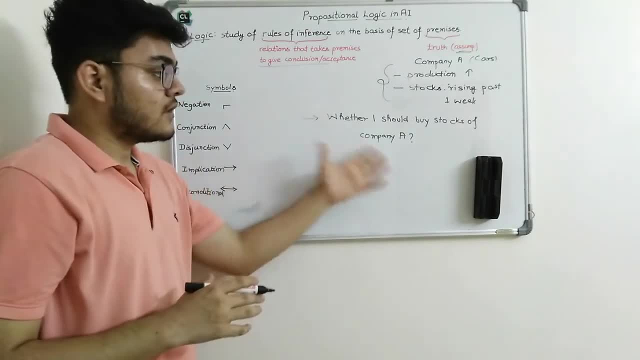 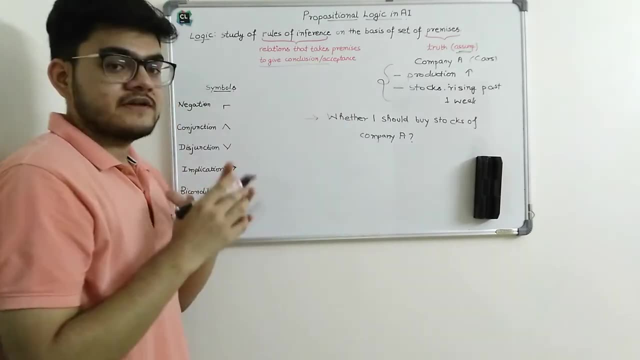 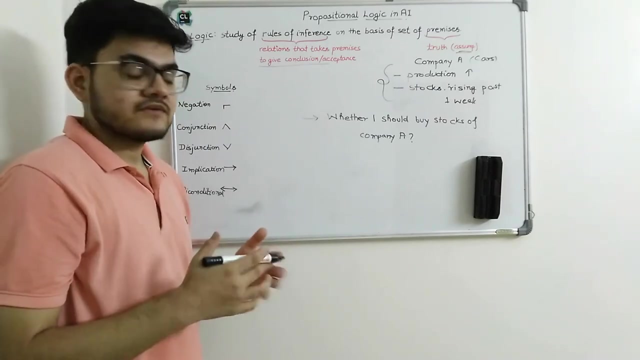 Propositional, predicate logic And a lot of things. So it is crucial that you Understand this definition here. Now, logics are of Different types, right? There are mathematical logic, Propositional logic, predicate logic, Formal, informal logic. 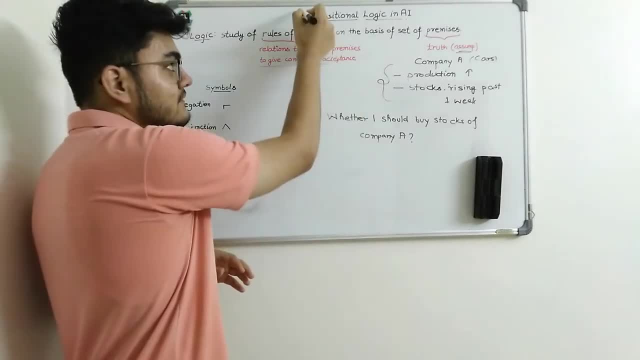 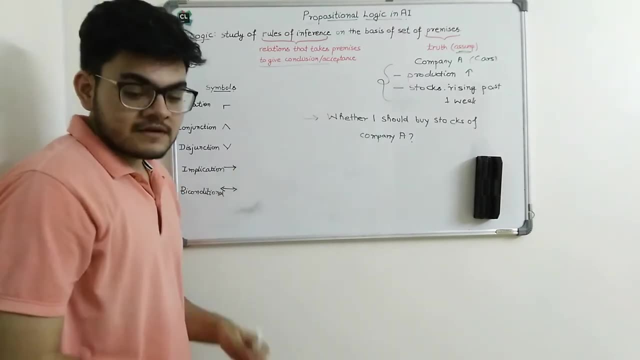 There are various types of logic In AI we are going to concern. We will be concerned about propositional logic And predicate logic. In this tutorial I am just going to cover The propositional logic. What is a propositional logic? Propositional logic: 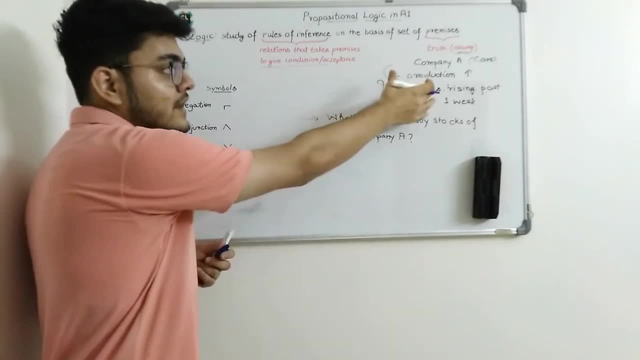 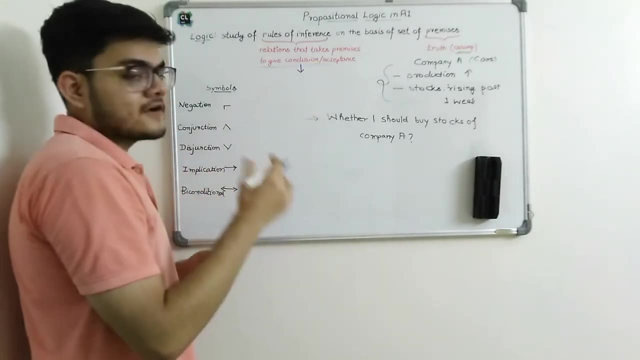 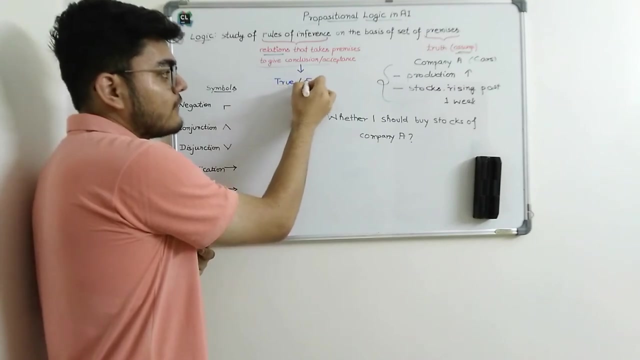 Is also just a same logic. It is going to have some Premises And some rules of inferences, But the conclusion That will come out of these Relations or functions Is going to be either true Or it will be false. 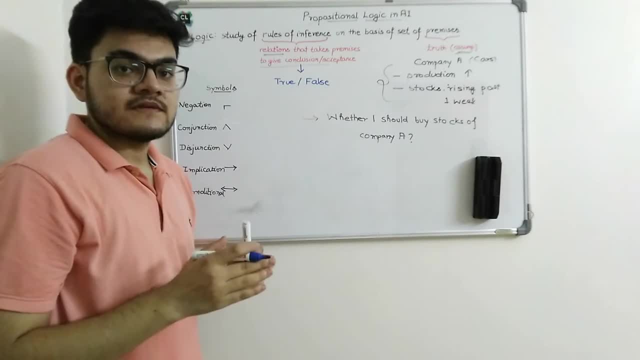 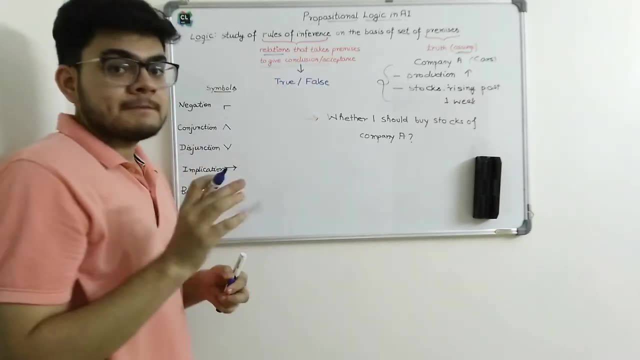 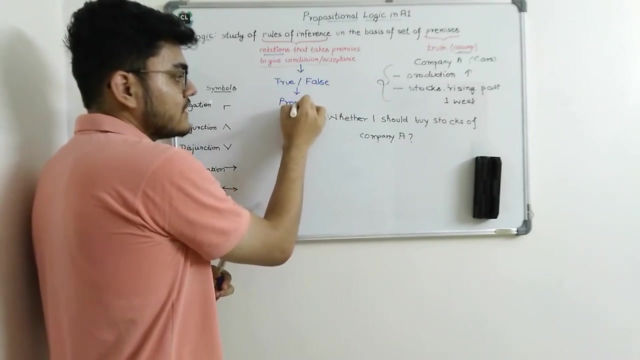 Right, True or false. If let us say The conclusion can be true or false, Then we can say that It is a propositional logic. So if it is true or false, I can say that it is a Propositional logic. 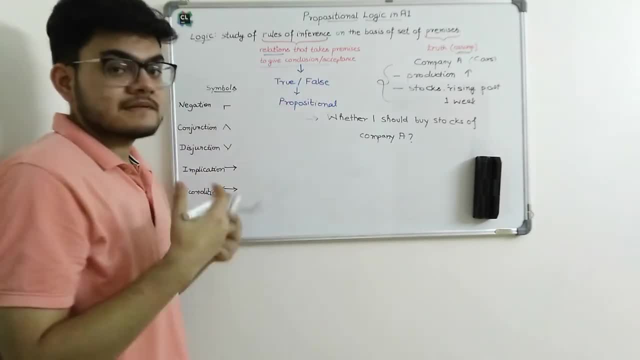 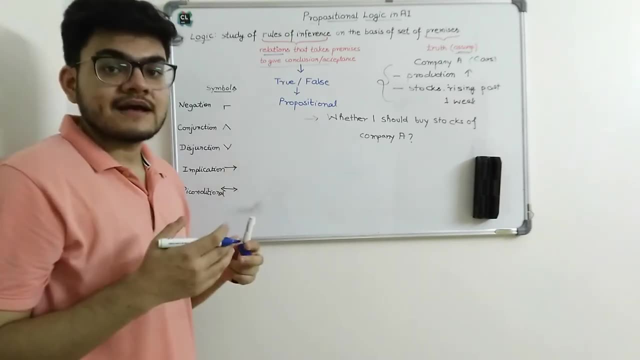 If it is, Let us say, if there is some conclusion Where it can be true And it can be false also, We do not call it as a proposition, We call it as a paradox. So if, let us say, I give a very simple statement. 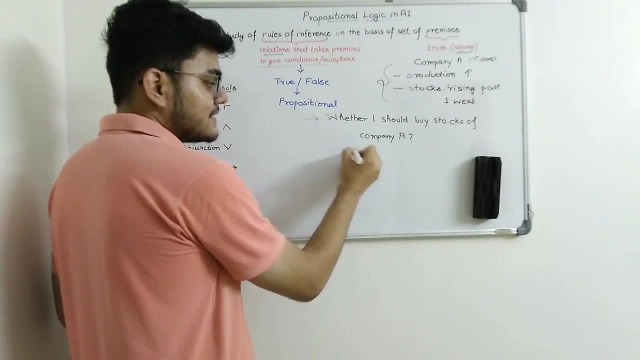 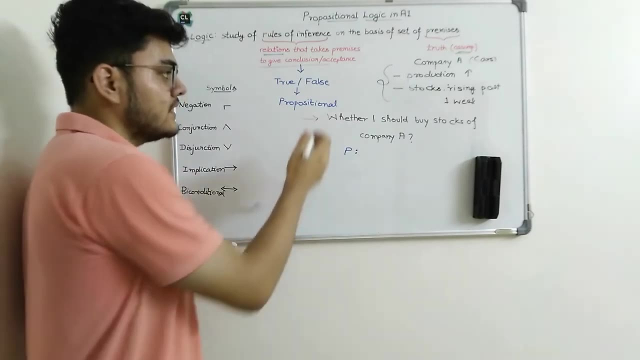 Let us say there is a statement. I will mark this statement as P. Right? I am going to say that. Let us take some example of propositional logic. So a proposition is true or false, Right? So let us say 2 plus 2 is equals to 4.. 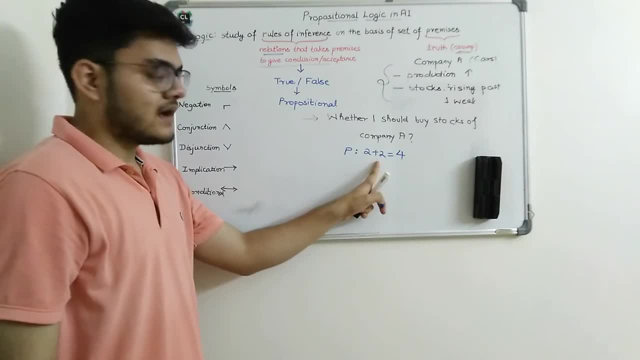 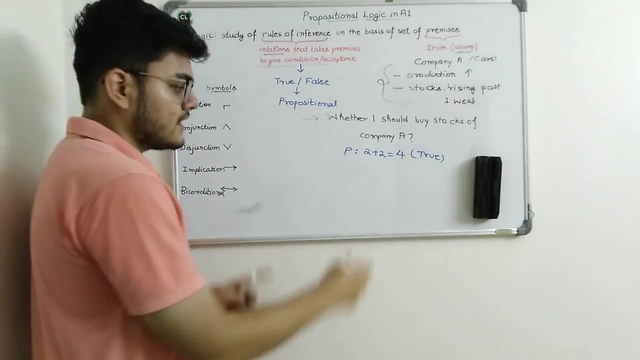 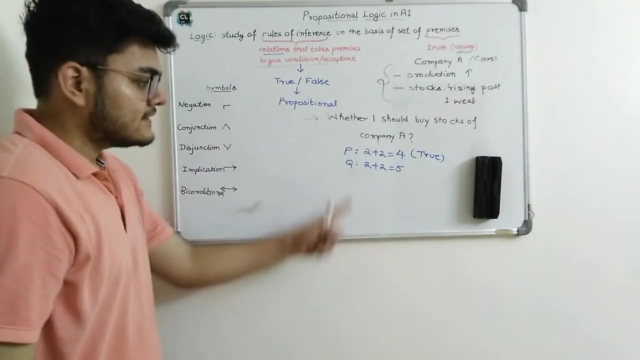 So is this a proposition? The answer is yes. Why? because This statement will evaluate to be true. Right Now I have another statement, Which is Q. Let us say 2 plus 2 is equals to 5.. Is this a proposition? 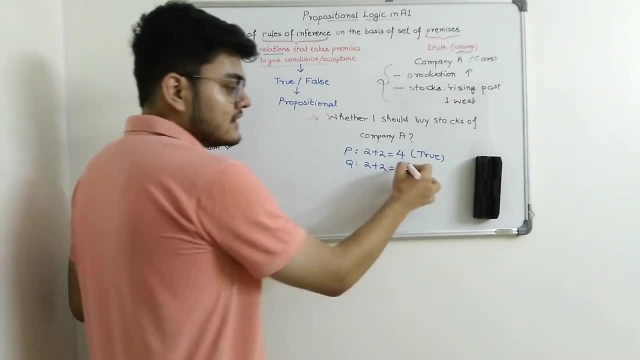 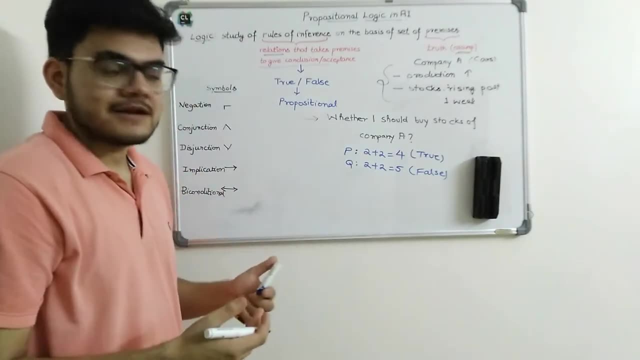 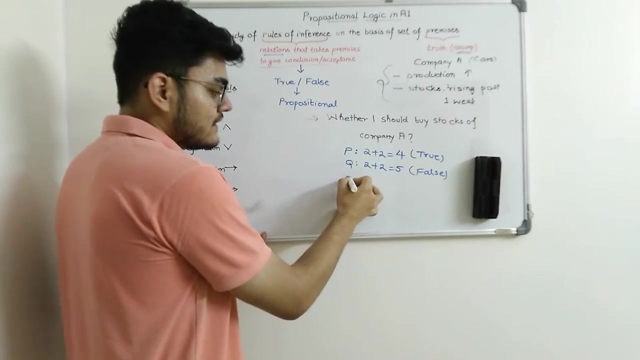 Yes, This is also a proposition, because This is false Right. So whatever statement you will have, It does not need to be a mathematical statement. It can be some other statements also, like Is it raining today, Or some questions Are not included in propositions. 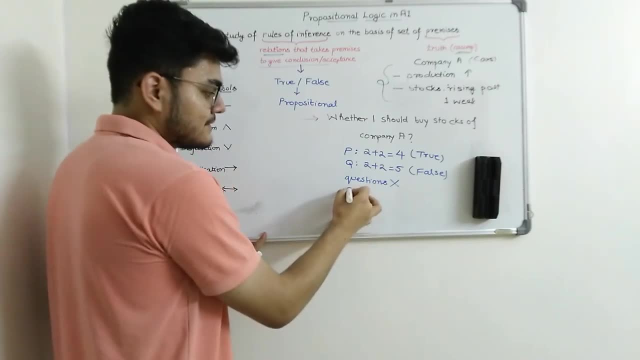 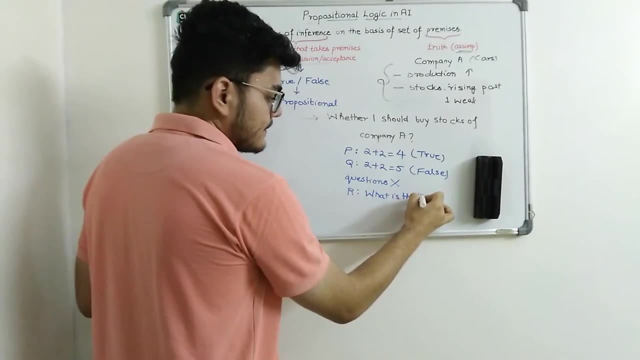 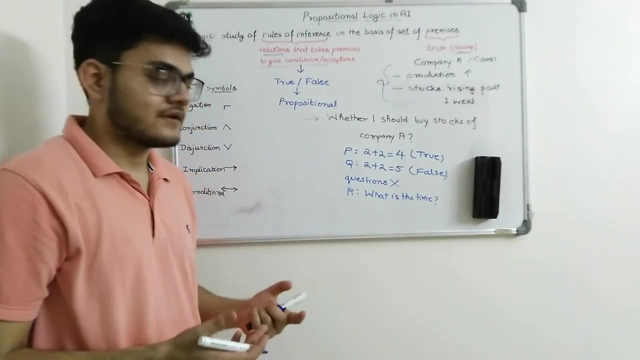 Right. So if someone, let us say, there is a Statement that Says: What is the time Right Now, this statement is neither true It is not false. So it is just a question, So it is not a proposition, Right? 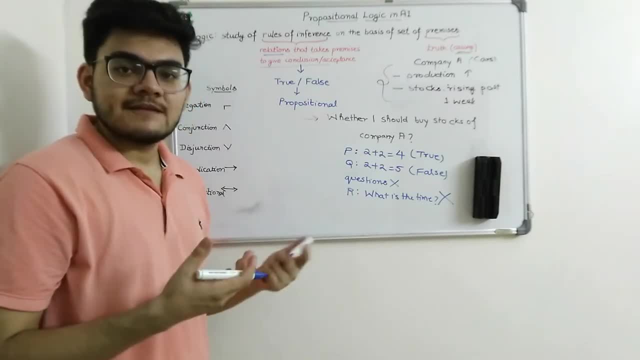 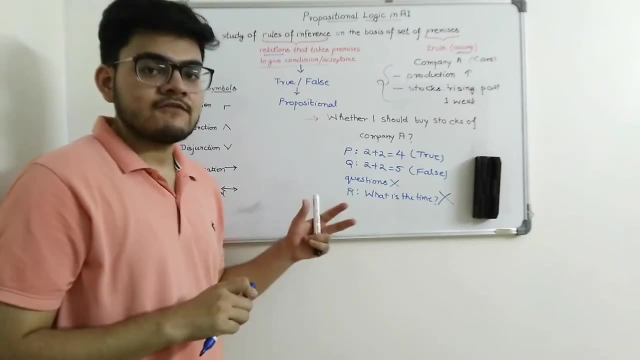 So this is not a proposition. So basically, propositions are statements Which are either true or they can be false. They can be mathematical statements Or some real life statements also. So let us say I say that I have 2 apples. I will say it is true. 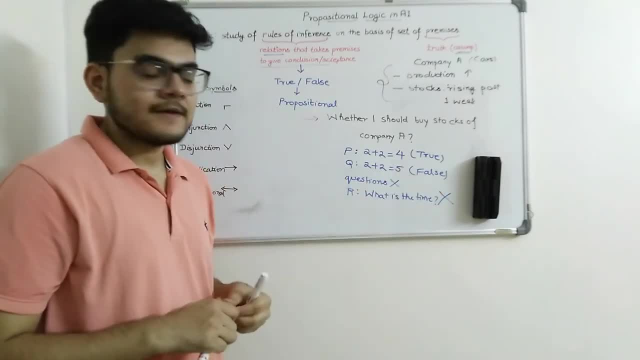 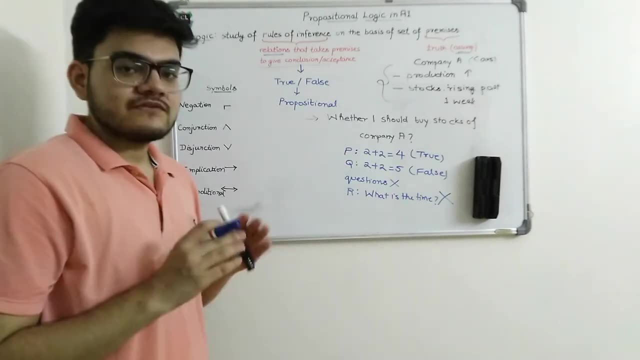 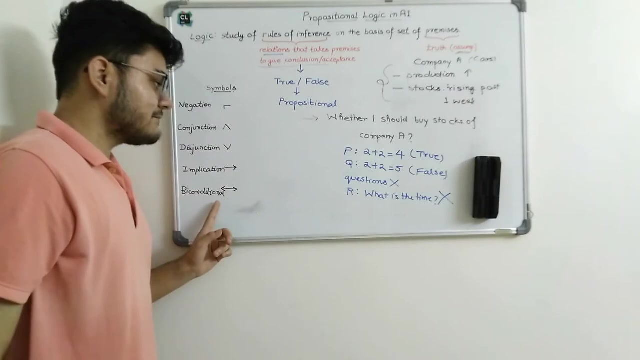 If I say that I do not have apples, It can be false also Right. So this way we derive propositions. Now, one important thing is That all the propositional statements, Or the propositional logic, Has 5 important symbols, Right. 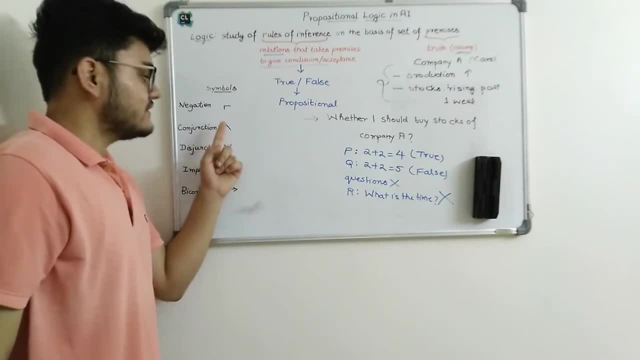 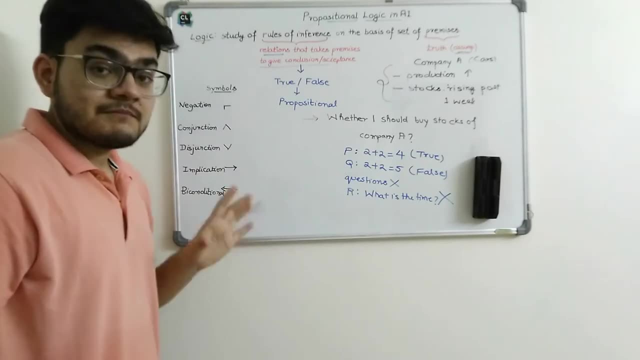 These are the 5 important symbols here which I have drawn. The first one is the negation, Conjunction, Disjunction, Implication and biconditional. So these are the 5 important symbols Of propositional logic. Using these symbols. 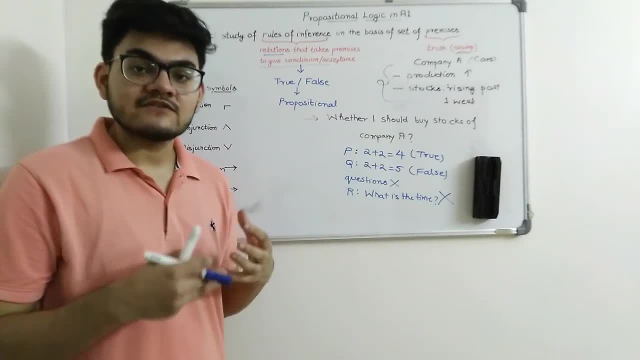 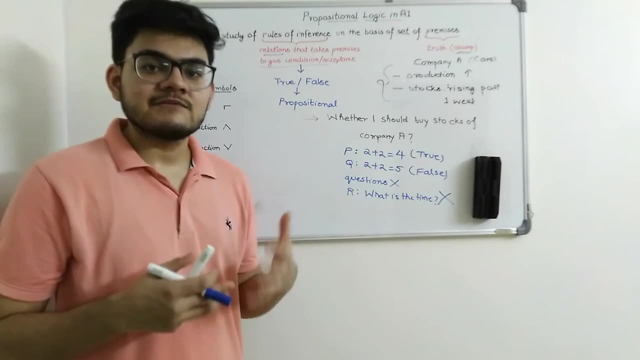 We can combine multiple statements And, using some logics and properties Of these operators, We can actually derive a logic out of these Right. So let us say I am given some statements, PEQRS, And let us say these statements. We will consider some examples. 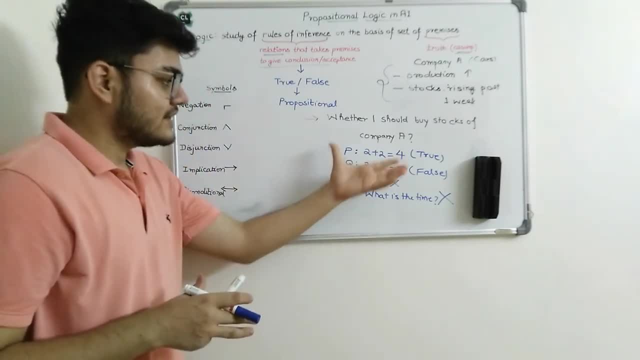 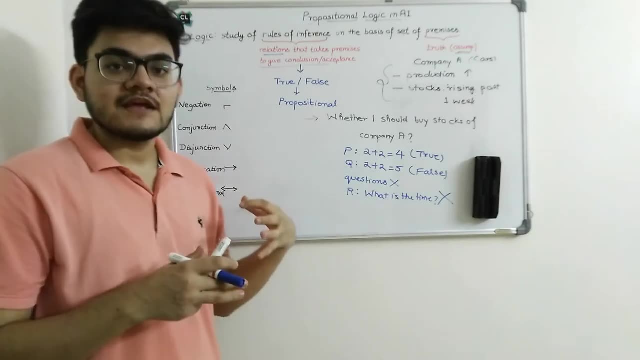 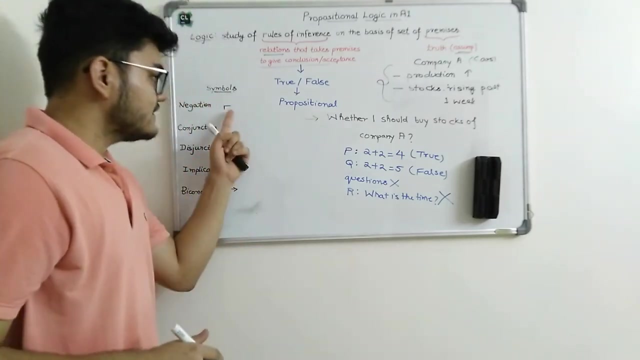 In the next tutorial also. Then we will study How we can actually take some statements, Apply these operators In propositional logic. We can say whether something is true or false. Right, Because that is the meaning, That is the essential meaning of proposition. 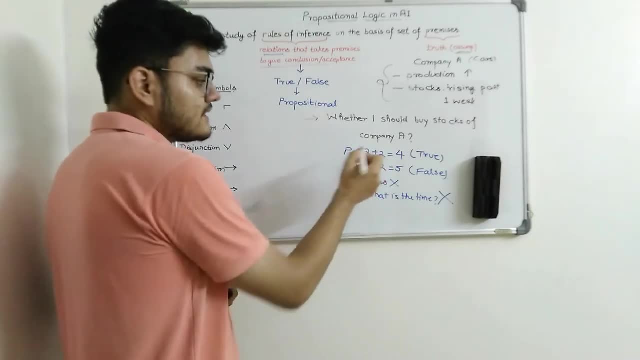 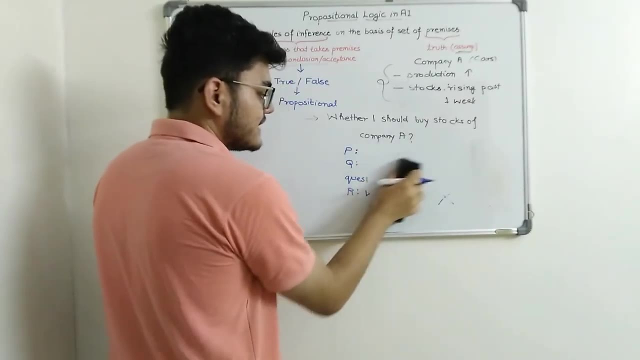 So let us study the first one, Which is the negation. So here you can see, We have a statement P. Let us take another statement. I am just going to remove this statement P, Right? So here I will take a statement P. 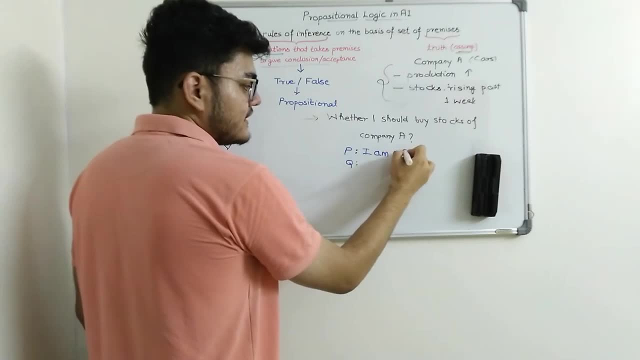 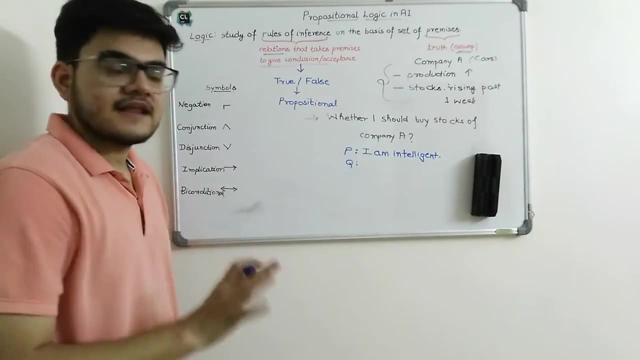 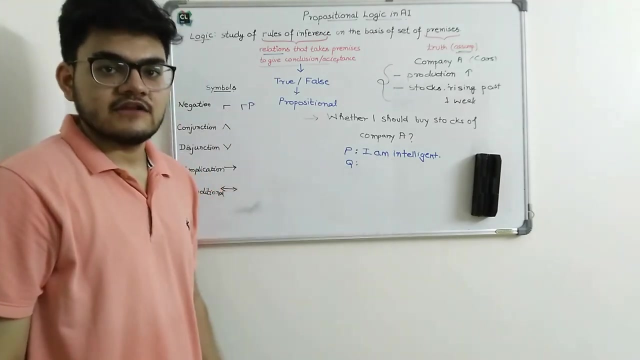 Which is: let us say: I am intelligent, Right? So this is A statement P, That I am intelligent. What is the negation of P? Negation of P means I am not intelligent, Right? So this is the meaning of negation. 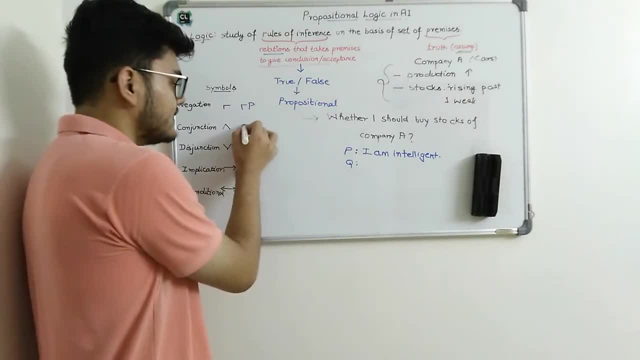 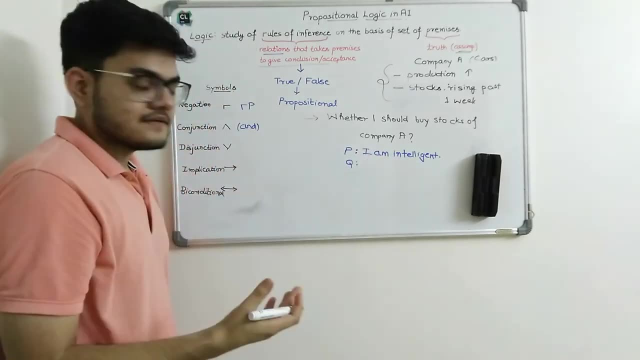 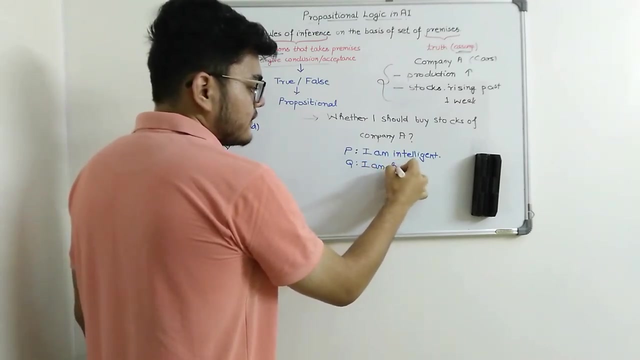 The second thing is conjunction. Conjunction basically means- and So I am just going to write here- And operator. So here I say I am intelligent. Let us take another statement, And here I will say that I am Hard working. 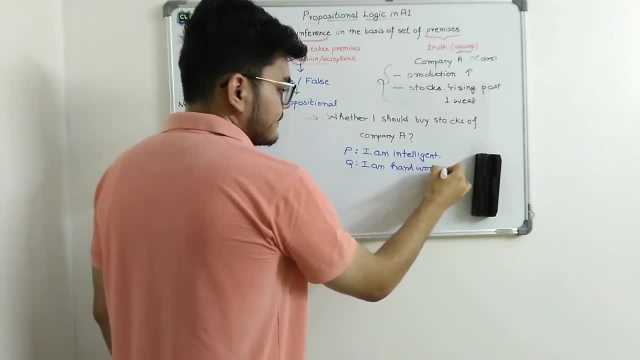 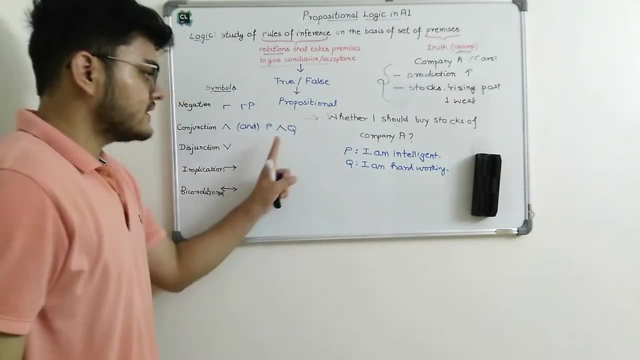 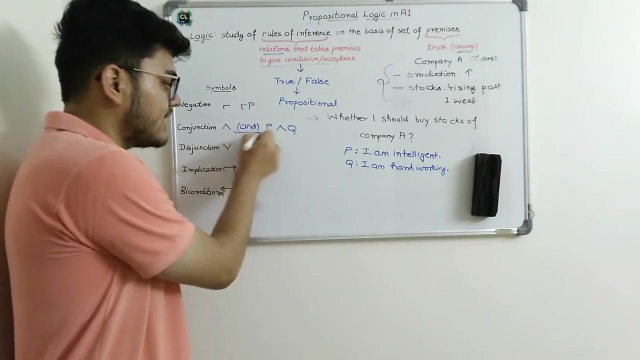 Right Now. if I say P Conjunction Q, What does this mean? This means that I am intelligent And I am hard working. So this conjunction basically means: and Now disjunction. If I say P, Disjunction Q, 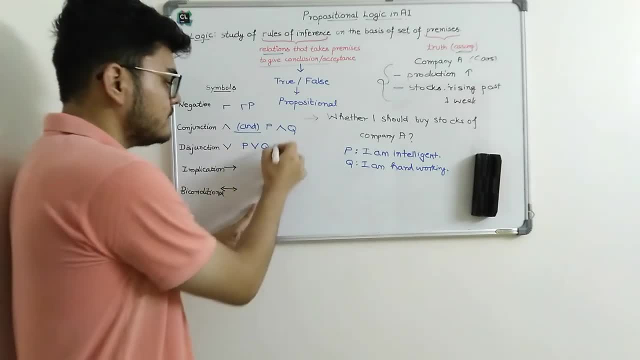 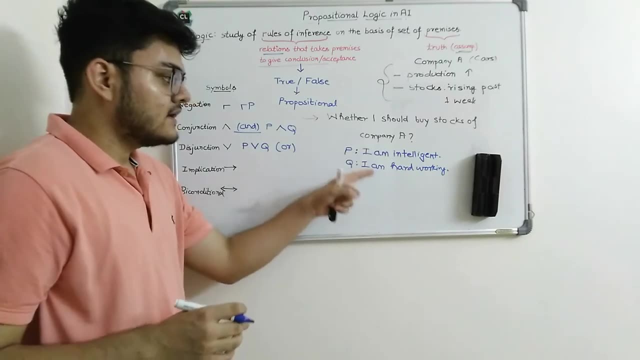 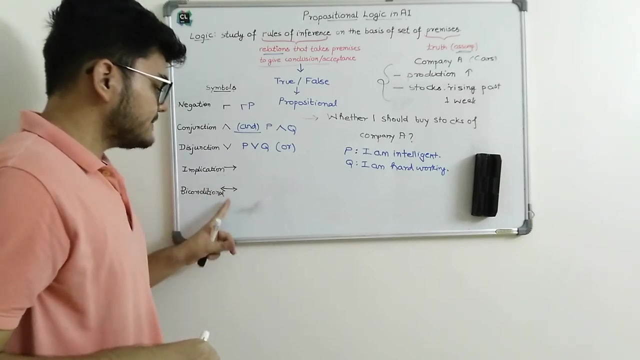 Or you can say P or Q, So it is similar to or operator, So I am intelligent Or I am hard working. One of them is true. Now we have implication. Right. Implication are of two types. One is single sided. 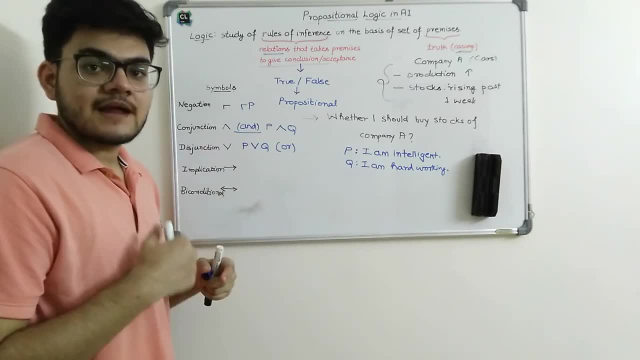 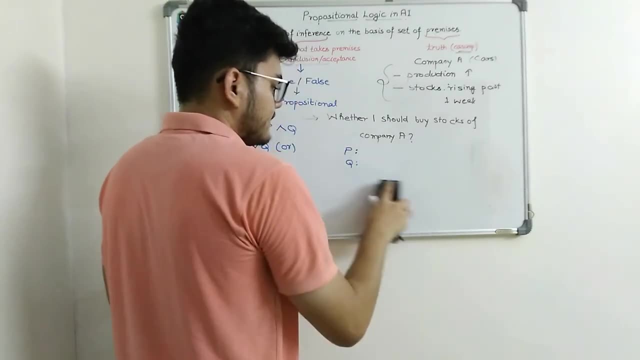 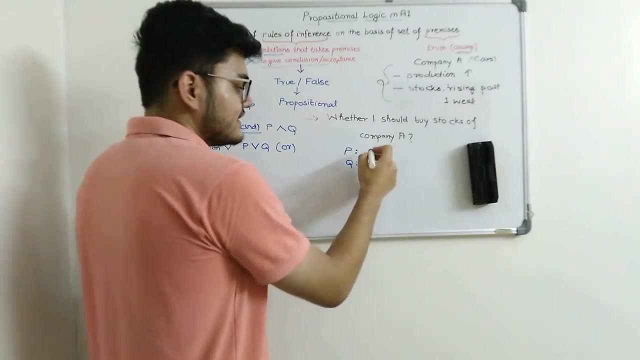 The second one is by condition, Which means both sides can be true. Right, So here I will take another example. Right, So here I will Say: In case of single implication, Let us take a very simple example. Here I will write: 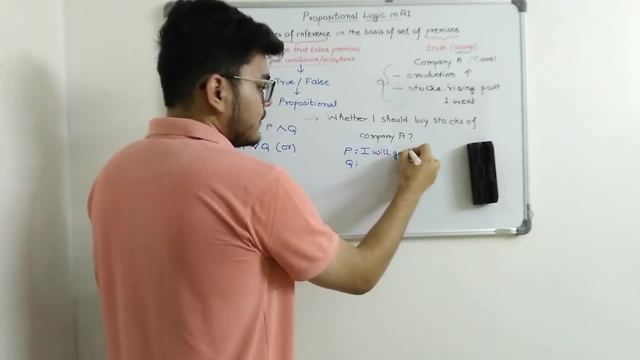 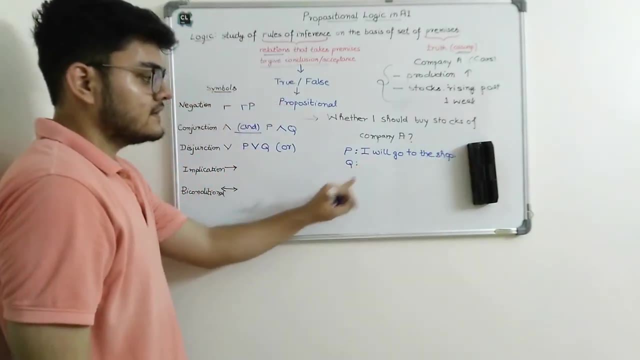 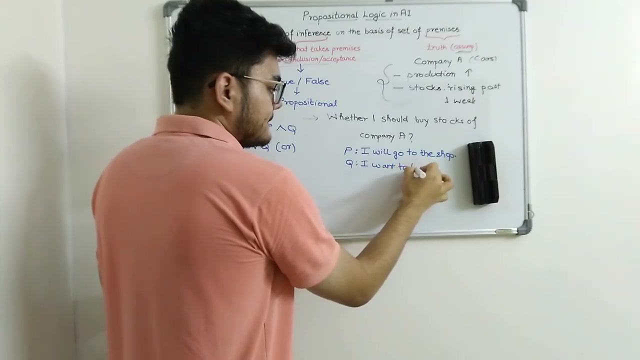 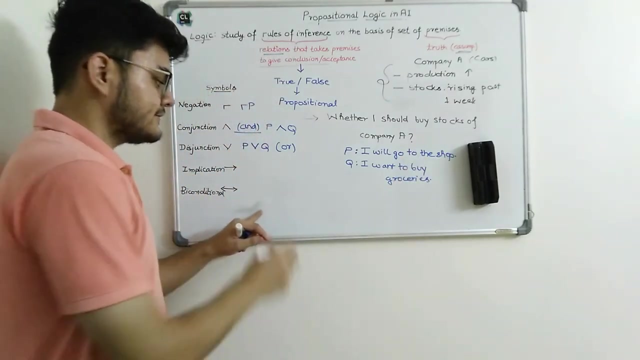 I will Go to the shop Right. This is the first statement. The second statement is Q- Right, Which is, I want to Buy groceries Right. So now I will write a Statement here: Q, Implication P. 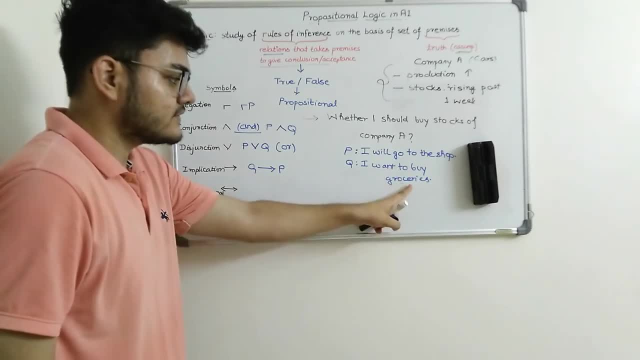 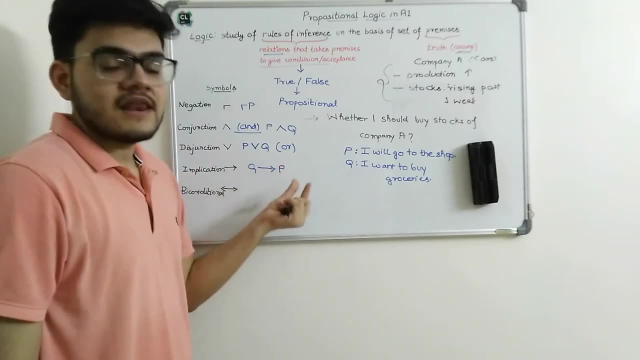 What does this mean? This means that I want to buy groceries, Which implies that I will go to the shop, Right? So if you want to buy the groceries, You will have to go to the shop. So this is single implication, Right? 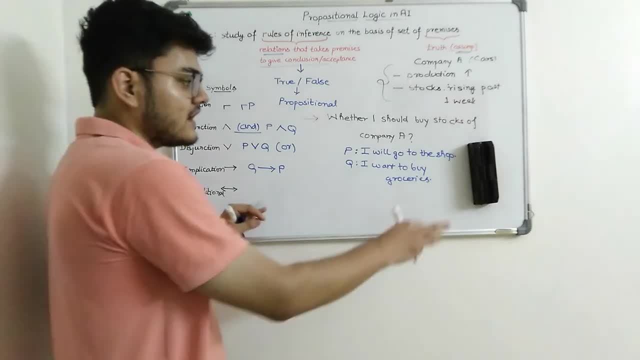 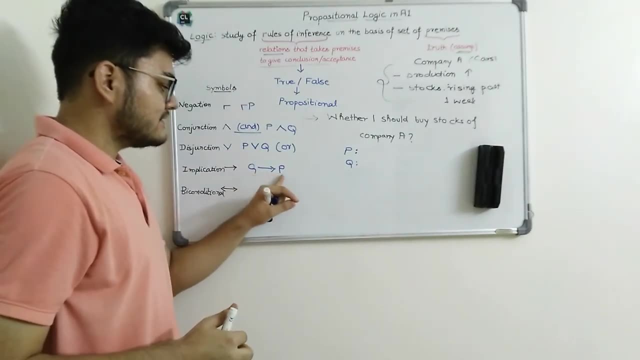 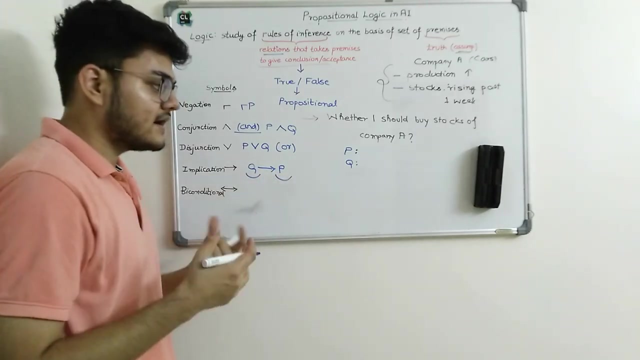 This implies this: Now we have double implication. I will take another example for that. You can even construct your own examples To understand this. So this means that, if this is true, This is implied Right. So that is the basic thing. 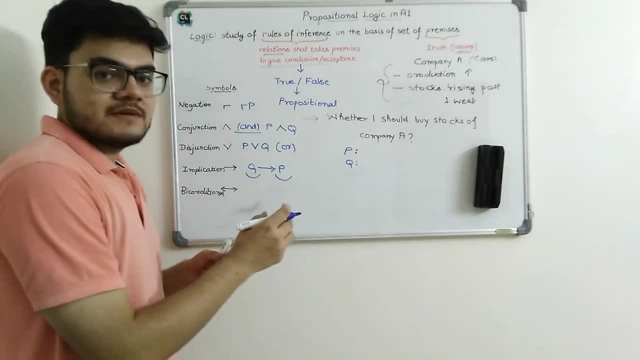 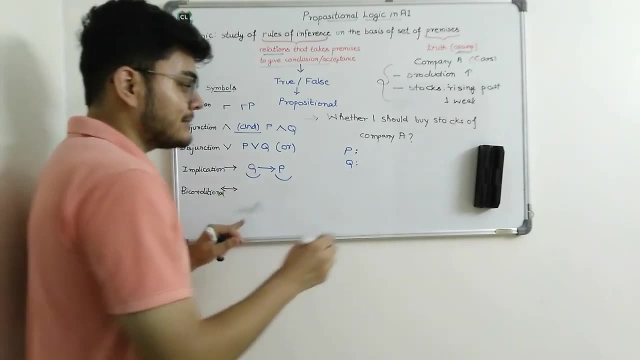 Now let us take a look at biconditional. Biconditional means both side is true, Which means that if one implies something, Then that second thing will also imply the first thing, Right? So let us take an example. So the first thing is: 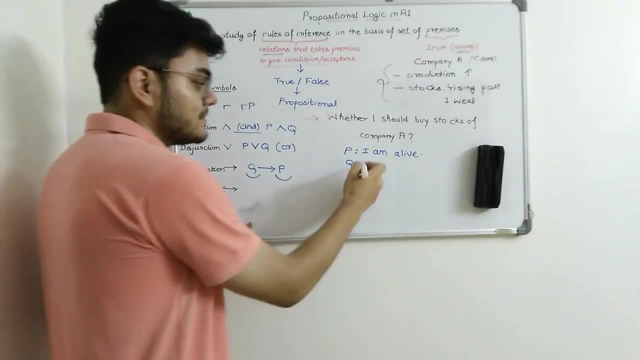 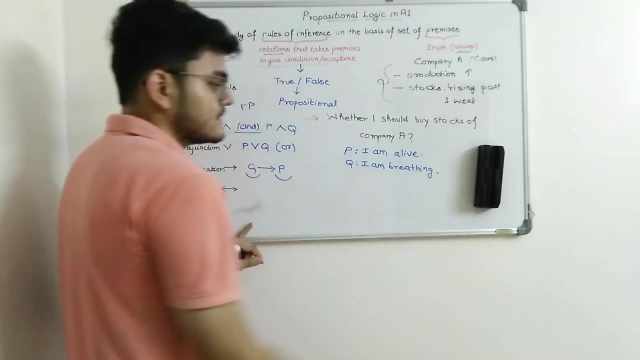 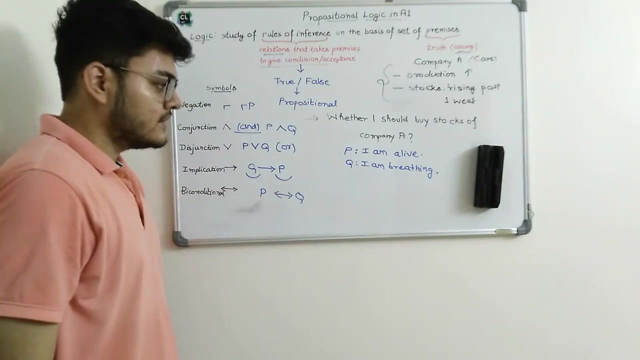 I am alive, Right, And the second statement says that I am Breathing. Now I say P, Double implication Q Or biconditional Q. So what does this mean? This means that P means I am alive, Which implies that I am breathing. 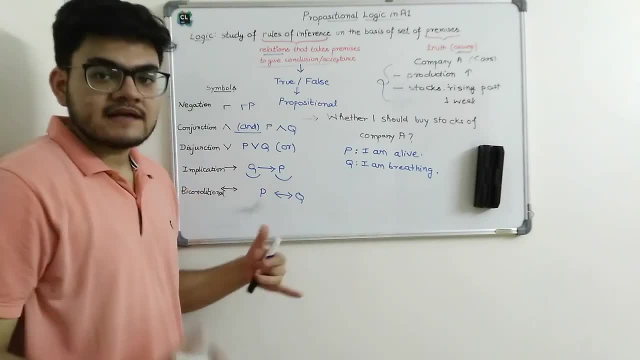 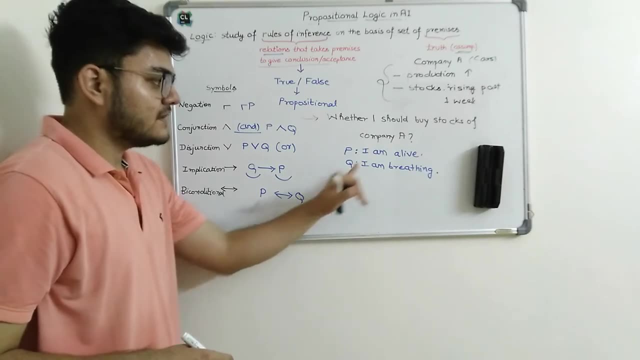 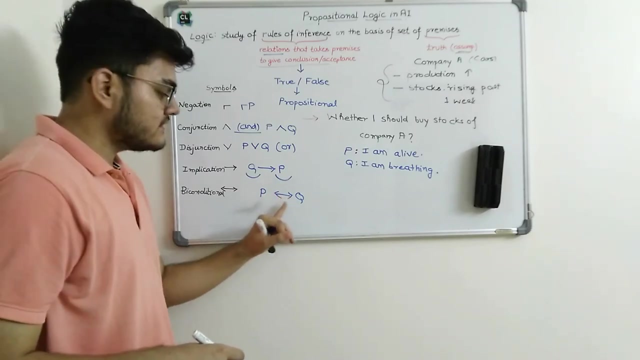 Right. So if I am alive, It implies that I am breathing. As a single implication first. So P implies Q, Which means I am alive, Implies that I am also breathing. Now just consider the opposite Right, Which is: Q implies P. 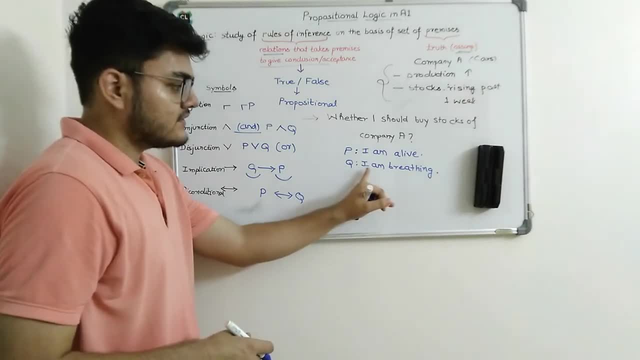 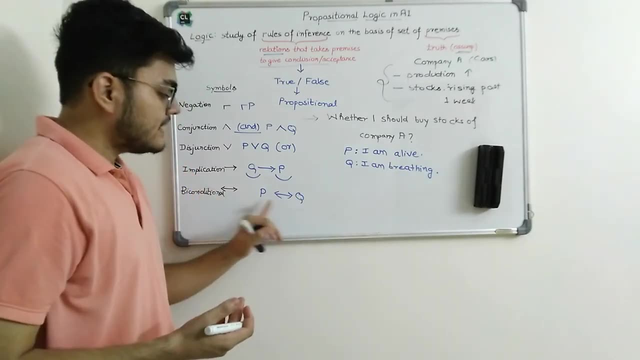 So is Q implies P true Right. So Q says I am breathing And obviously, since I am breathing, I am alive. So Q implies P is also correct. So P double implication Or biconditional Q means That if one statement is: